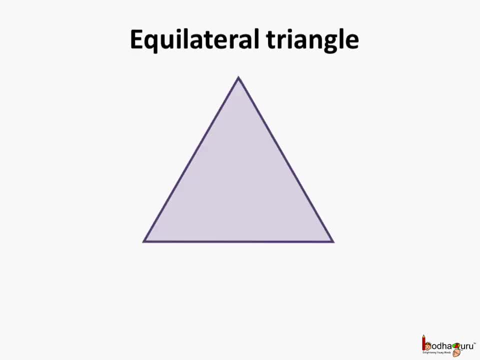 Now, in case of an equilateral triangle, all the three sides are equal, So we can say it is a regular polygon, Meaning a polygon which has all the sides of equal length. So we can say it is a regular polygon. An equilateral triangle is a regular polygon with three sides and its perimeter is equal to. 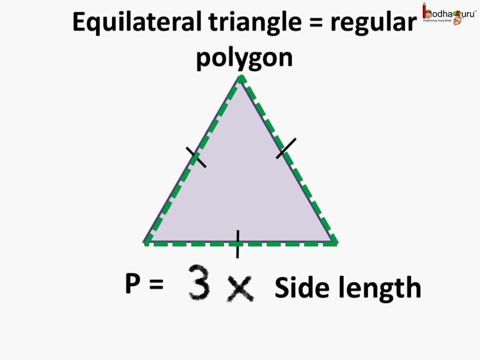 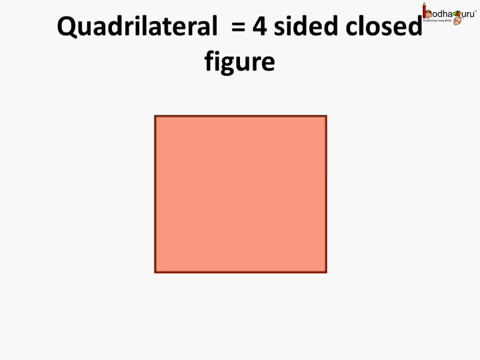 three times the side length, where all the sides are of equal length. Now if we come to a quadrilateral, then we know it is a four-sided closed figure. Now if all the four sides are of equal length, then we can say it is a regular quadrilateral. 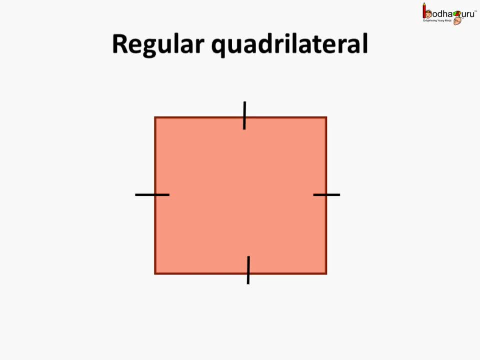 What is the perimeter of a regular quadrilateral? We can say it is equal to four times the side length, as it has four sides of equal length. Now here we have a closed figure with one, two, three, four, five sides, So it is a pentagon with five sides. and if all the five sides are of equal length, then 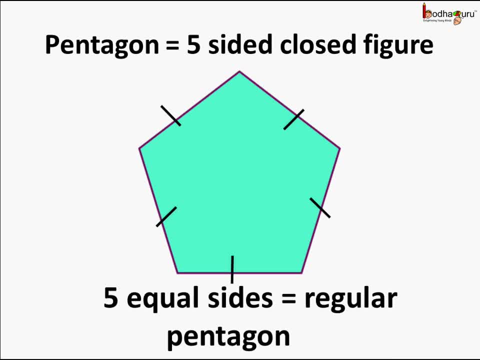 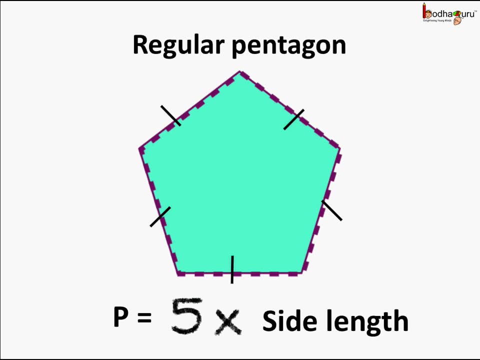 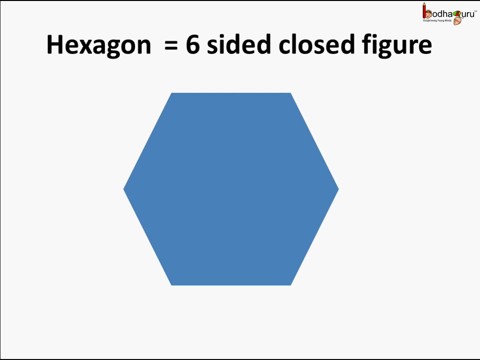 we can say it is a regular pentagon. Now, what will be the perimeter of regular pentagon? It will be equal to. it will be equal to five into the length of each side, Which is same for all the five sides. Next, if we think of hexagon, then it is a six-sided closed figure. 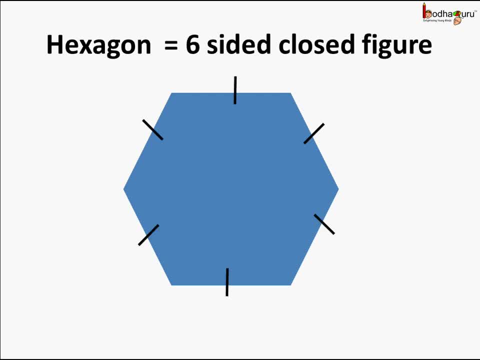 And when all the sides are of equal length, Then we can say it is a regular hexagon. So a regular hexagon is a hexagon which has all the six sides of equal length. Here what will be the perimeter? As we can say, all the six sides are of equal length. 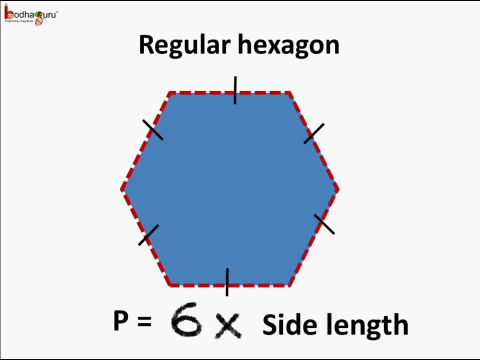 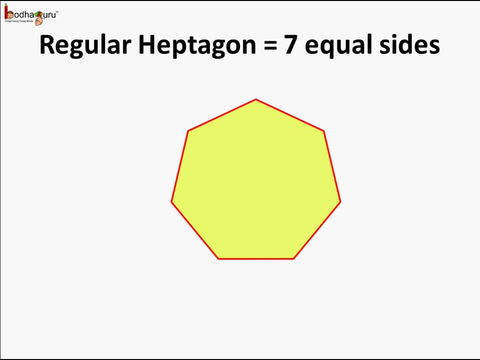 Perimeter will be equal to six times the length of each side. And what about heptagon? A heptagon is a seven-sided closed figure, And if all the seven sides are of equal length, then we say it is a regular heptagon. 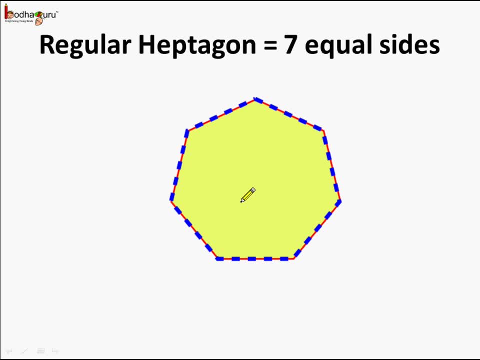 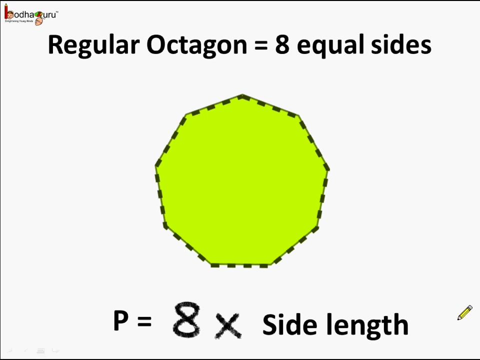 And the perimeter in this case will be equal to seven into the side length. We can say in an octagon There are eight sides And when the length of each side is equal Then it becomes a regular octagon And the perimeter of regular octagon will be equal to eight times the side length. 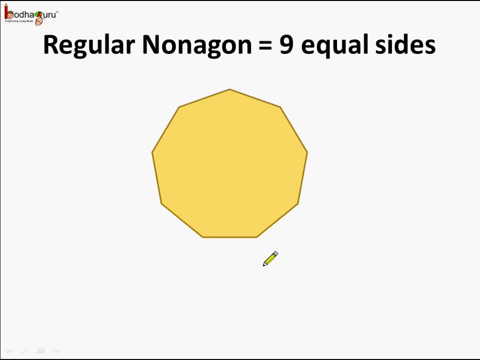 Same way, when a closed figure or a polygon Which has nine sides, it is called a nonagon, And when all the nine sides are of equal length, Then we can say it is a regular nonagon. And what will be its perimeter? Its perimeter will be equal to nine times the side length. 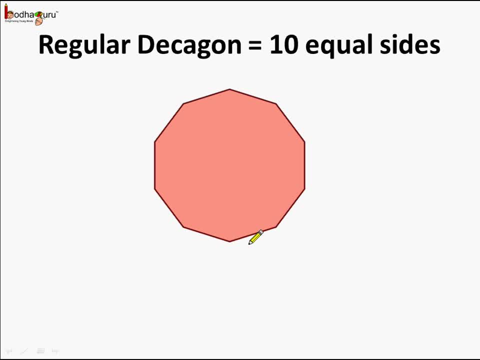 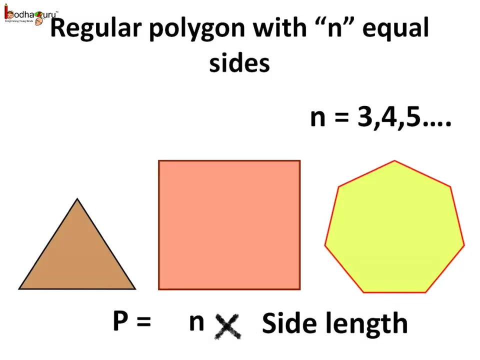 Same way, we come to a figure with Ten sides, And when all the ten sides are of equal length, It is called a regular decagon, And the perimeter will be equal to ten times the side length. So what did we see? That any regular polygon with n equal sides. 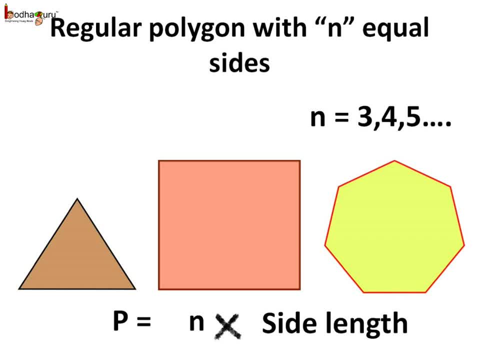 Here n can be three, four, five and so on. If you remember. it cannot be two or less than two, Because then we won't get a closed figure, And the perimeter of all these regular polygons With n equal sides will be equal to.